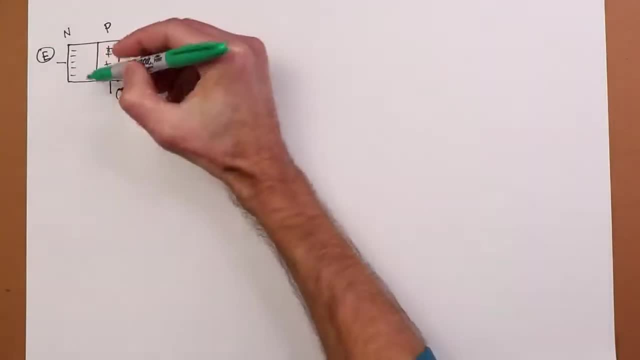 depleted of free charge. So we have a depletion region here and we have a depletion region here, And so, with diodes, that creates an energy hill. All right, how does this little configuration work? Well, if you look at this sort of simplistically, 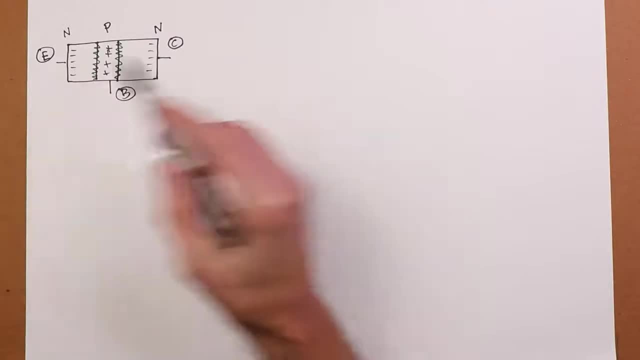 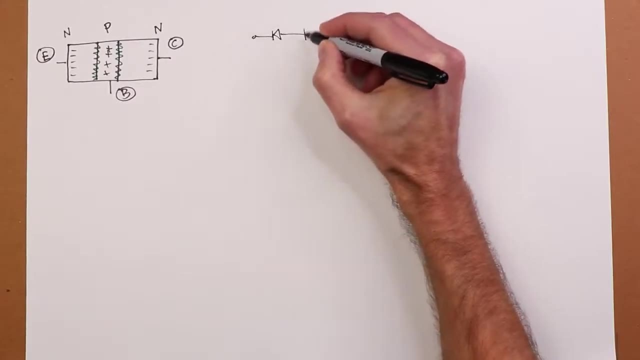 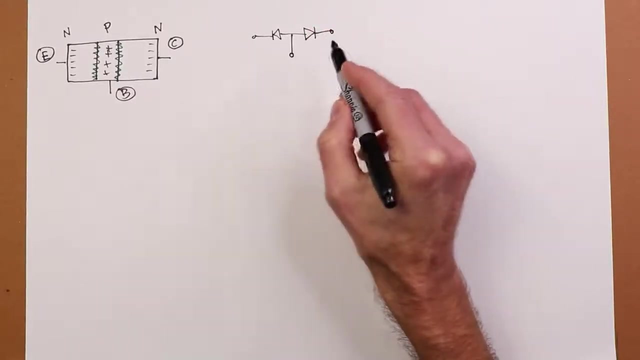 you might say: well, look, that's PNPN, Isn't that like a diode? In other words, you might think to yourself: well, that's basically this. All right, you've got your NPN, You've got the NPNP and PN junctions. Is that the same thing? Well, in some cases it can in fact be. 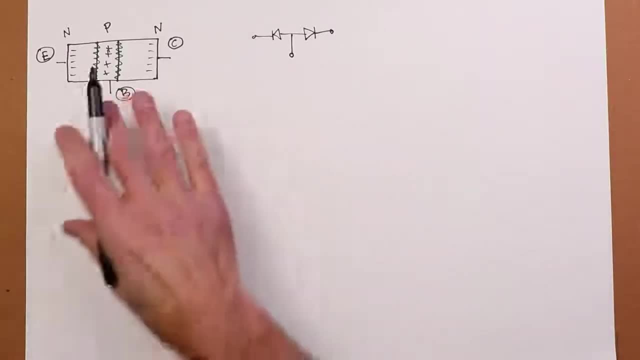 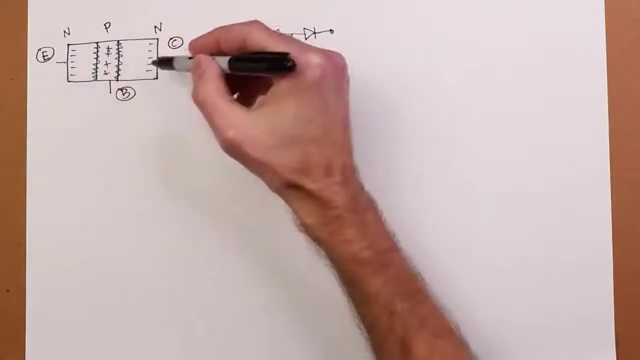 analyzed that way, But there's a very important distinction. All right, the fact that this P material is contiguous. It's not like it's a piece of P material and a wire and another piece of P material, which is what we're talking about here. 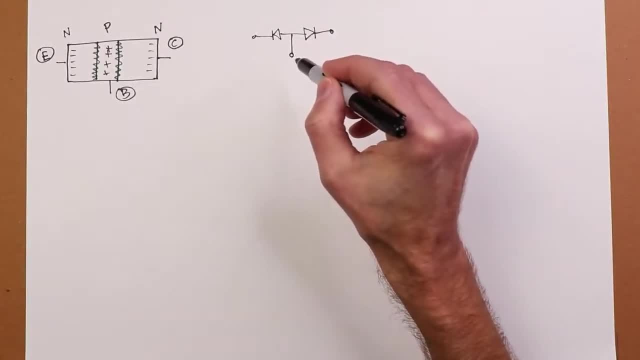 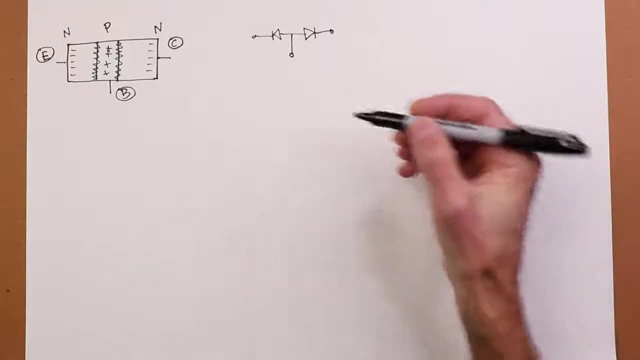 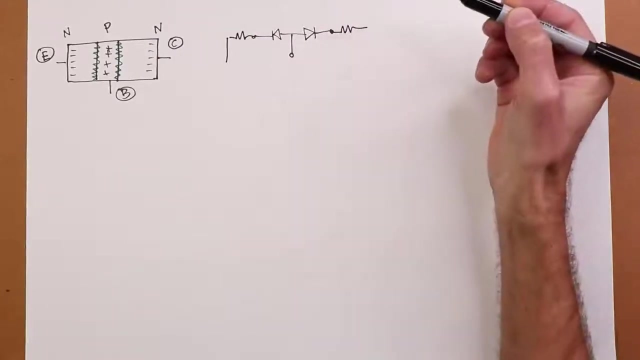 But this is actually useful in terms of explaining, at least partially, how this thing is going to work. So what we're going to do is attach a couple of power supplies and some resistors, Basically some current limiting resistors over here. Now I have options on my polarities for 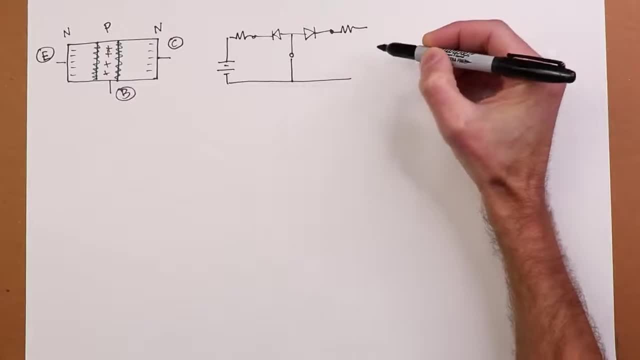 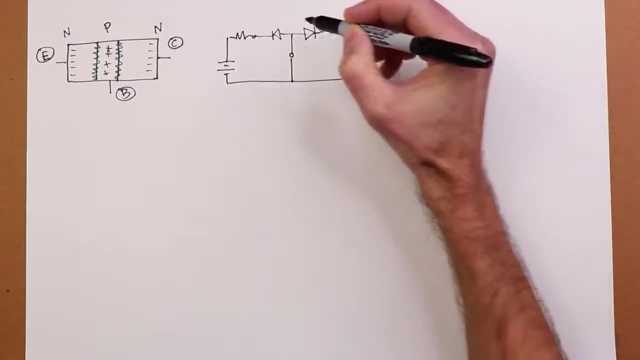 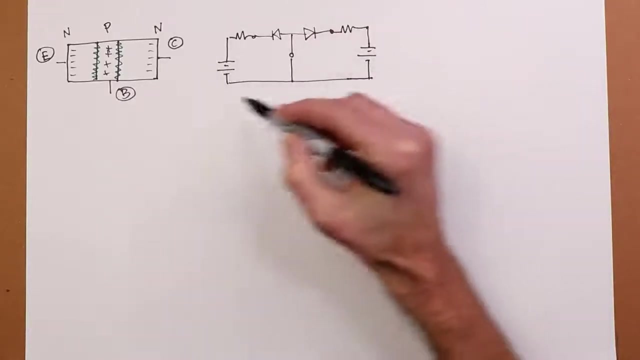 my sources. So I'm just going to set this up like so Right now. again: emitter base, collector. So this would be our emitter power supply, This would be our collector. power supply Base would be at the common point here. Now look at the polarity of these two power supplies. They reverse bias. 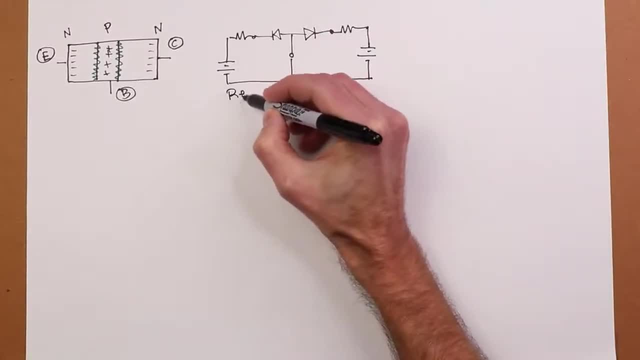 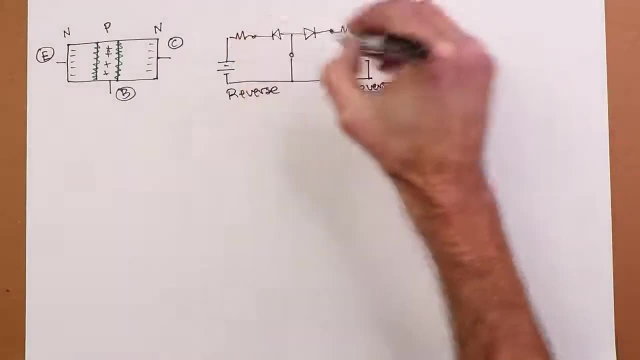 these diodes Right. so this is a reverse bias. This is a reverse bias in these two loops Right, this loop, this loop. What ends up happening? Well, current in both sides, in other words, in the emitter side and the collector side. 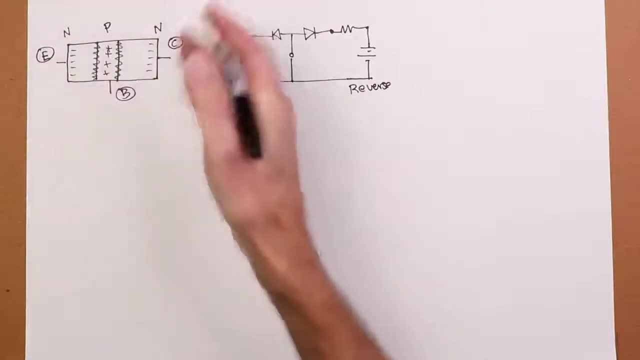 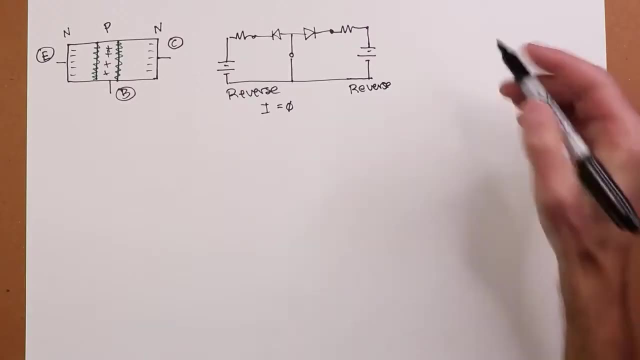 is zero. And if you take an actual BJT and you hook it up like this, that's exactly what's going to happen. Okay, what happens if we do the opposite? What if we flip the power supplies? So if we do the opposite, it's going to be a negative. 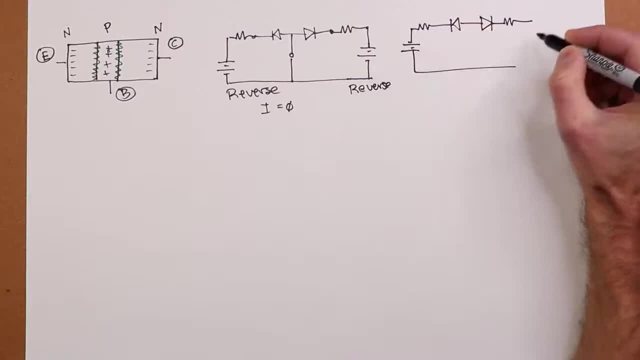 So make this guy negative. Now, what do we see? Well, these are both forward biased. And if you wanted to figure out the individual currents, right, you know, here you've got a loop like this, here you got something like this: 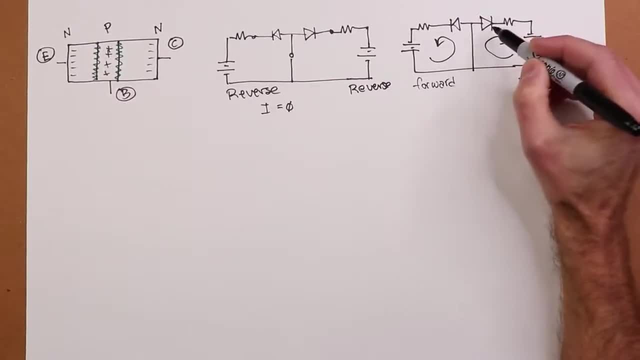 you would take your power supply, subtract the forward drop on the diode- 7 tenths of a volt if it's silicon- and divide that by your current limiting resistor. So, for example, this current over here would be this power supply. Let's just 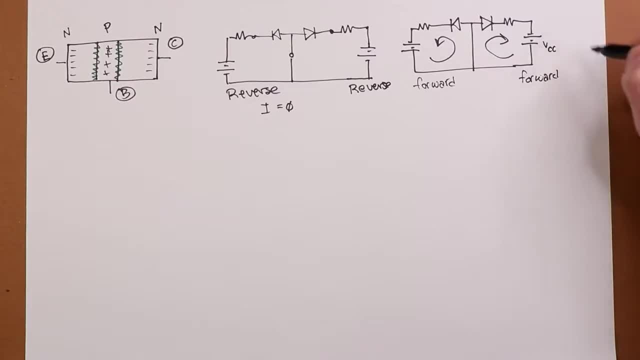 we'll call that VCC for collector power supply. So this current would be VCC minus approximately 0.7 volts for the diode and that would be divided by this resistor. We'll call that the collector resistor. That would get you the current. Same thing would happen over here. 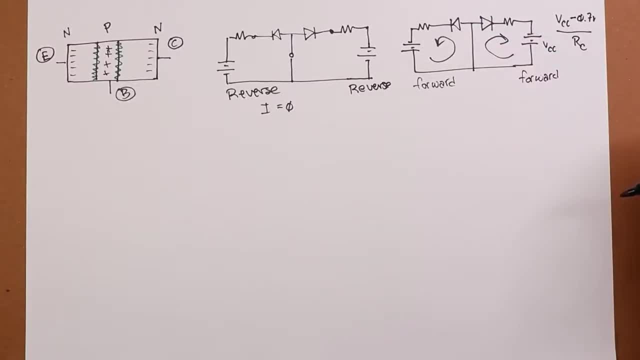 on the emitter side. All right, so what happens if we have one forward and one reversed? Okay, now you might expect a small current on one side and a large current in the other. In fact, that doesn't happen. Something entirely different happens. 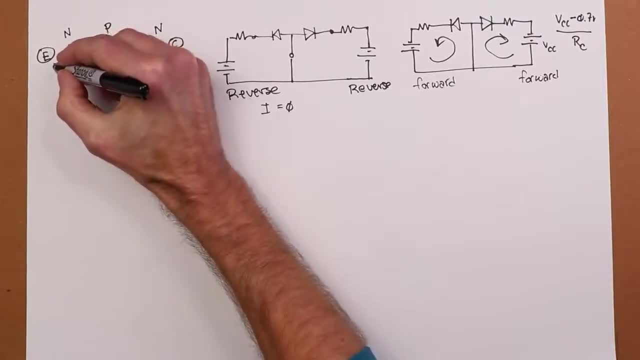 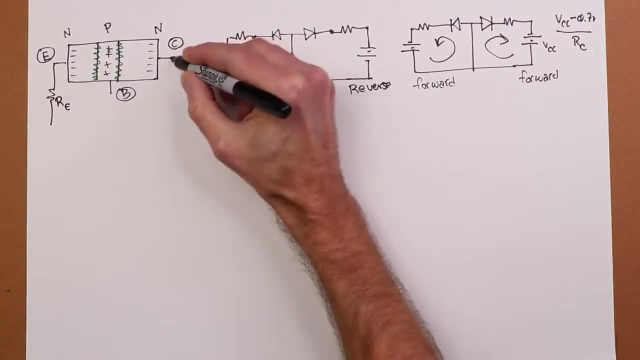 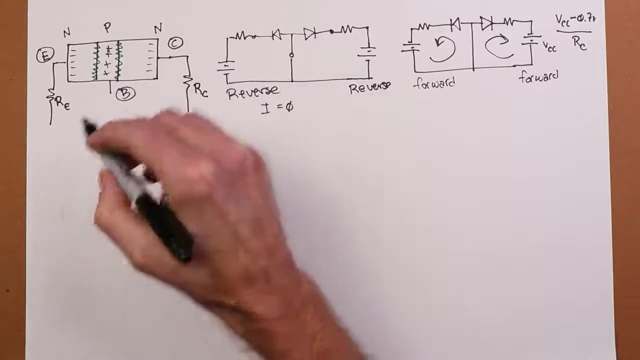 Let's take a look at our original circuit back here. So I'm just going to add our resistors. I'll call this the emitter resistor, like I did over there. This will be the collector resistor and I'm going to set that up so that I have a forward. 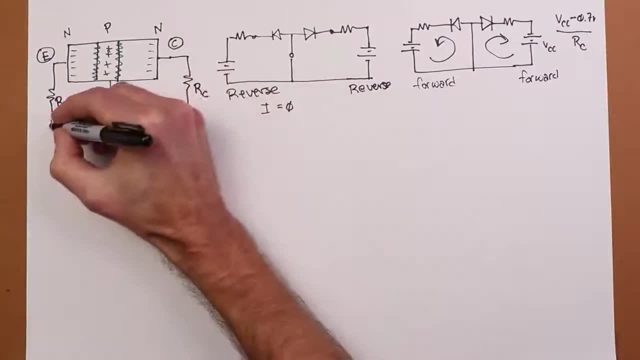 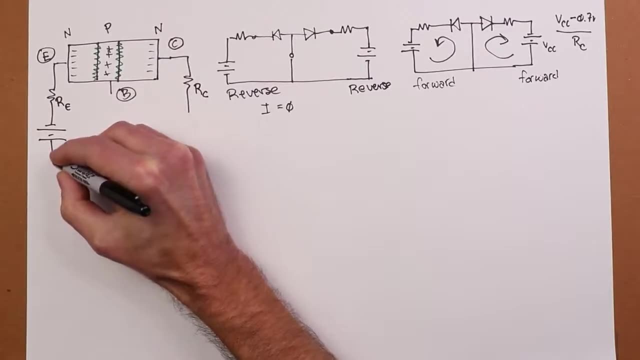 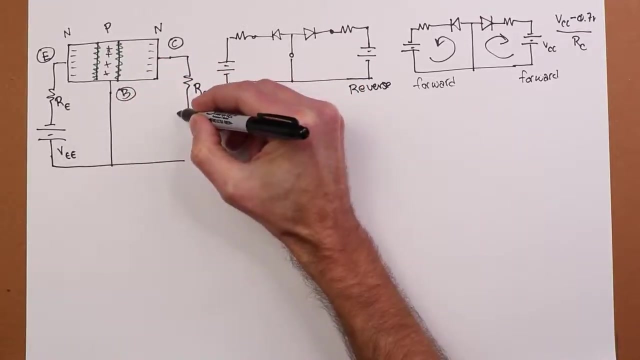 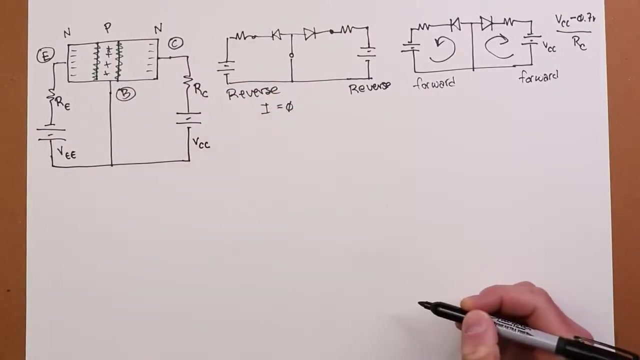 bias on this side and a reverse bias on this side. So here's my emitter: power supply VEE Base is going to come straight down and then over here we'll have our VCC, Alrighty, Okay. so again, this is forward biased. 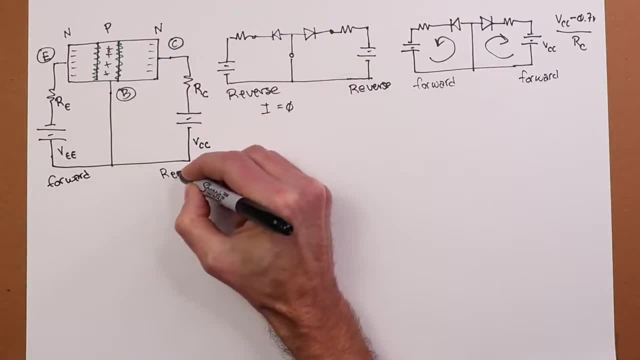 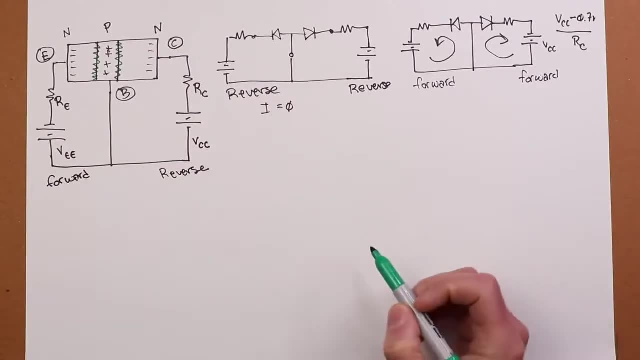 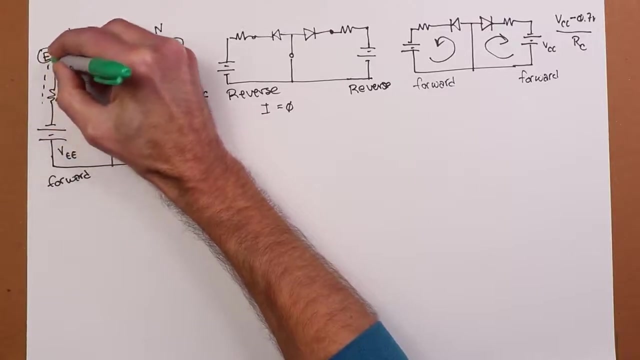 This junction, the collector base junction, is reverse biased, So to make this a little bit more obvious, I am going to use electron flow here. Here's what ends up happening on the emitter side. The electrons are going to leave the negative terminal. They enter the end material, where they are the majority carrier. 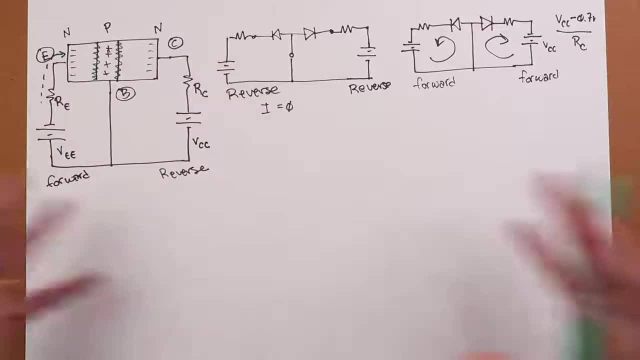 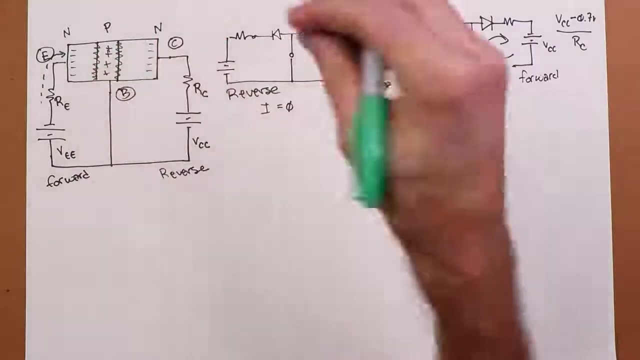 If there is sufficient voltage—in other words sufficient electrical pressure—we can hop the depletion region. The electrons wind up in the P base. Now some of those electrons are going to recombine. with the holes right, You can think of the electrons as force. They're going to recombine. 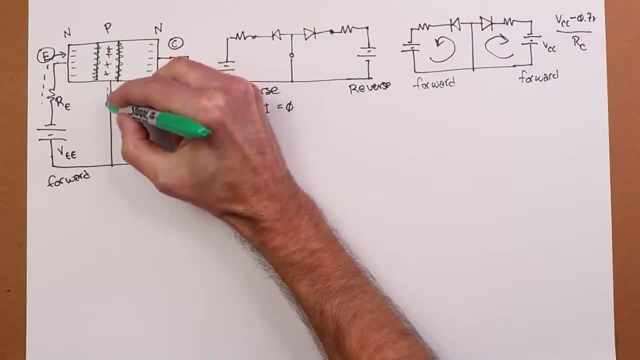 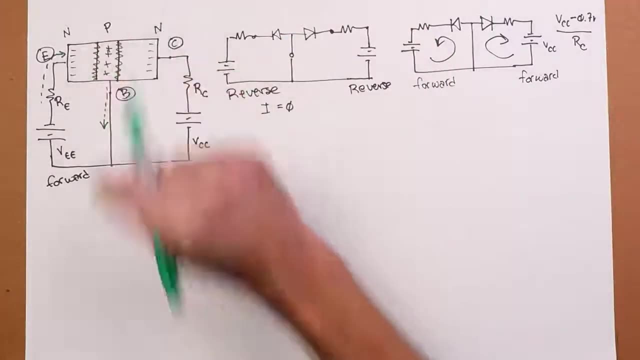 of dropping into the holes And that produces an exit current, sometimes called a recombination current, your base current. However, this region is thin and lightly doped and there simply isn't enough time for all of these electrons to fall into holes. The vast majority of them, maybe 98,. 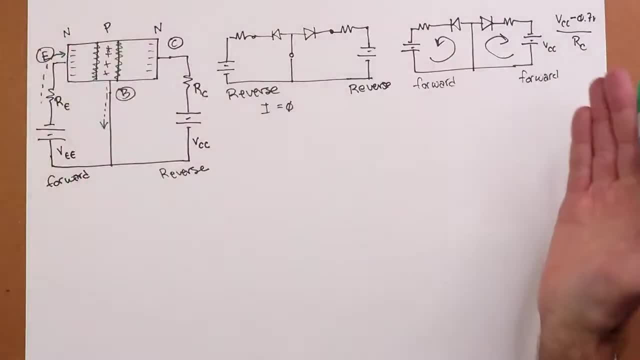 99-plus percent wind up going into the collector, where they're the majority carrier, and they will simply return back to the collector supply As percentages go. like I said, the vast majority goes from the emitter into the collector. The electrons are emitted into the emitter. 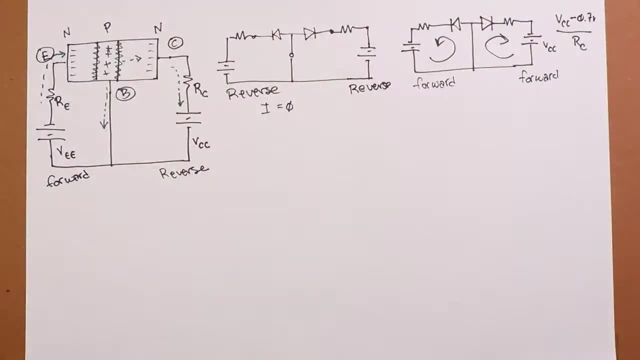 appropriately named and then they're collected back up at the collector. collector, and that's where the names come from. okay, so what do we see here? well, you know, some of the basic ideas are that. you know, Kirchhoff's current law must still be true. so ie would have to equal IC plus IB, right, that's just. 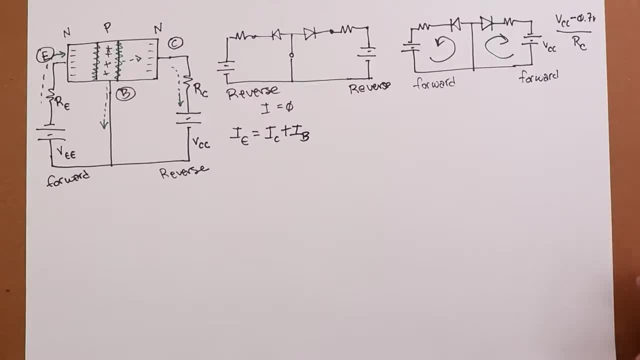 basic Kirchhoff's current law. but if this percentage is very close, right, if IC is, you know, 99% of ie, then you can say that the emitter and the collector currents are approximately the same size. okey-doke, now put some figures of merit on here. we talk about the percentage that 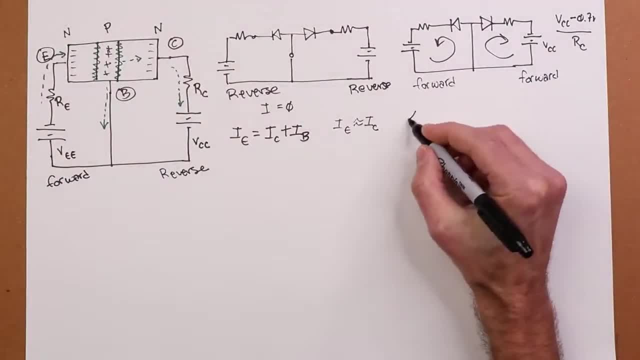 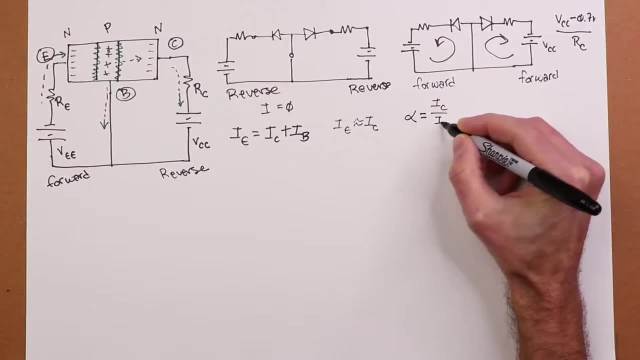 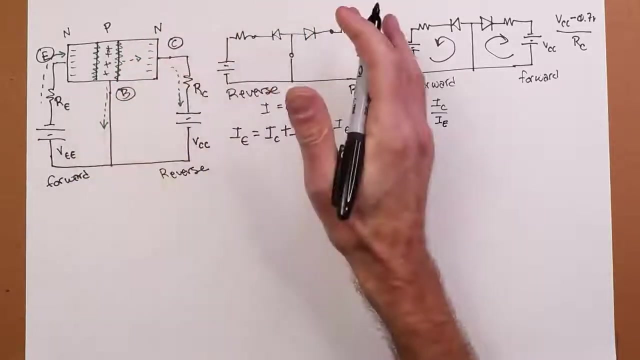 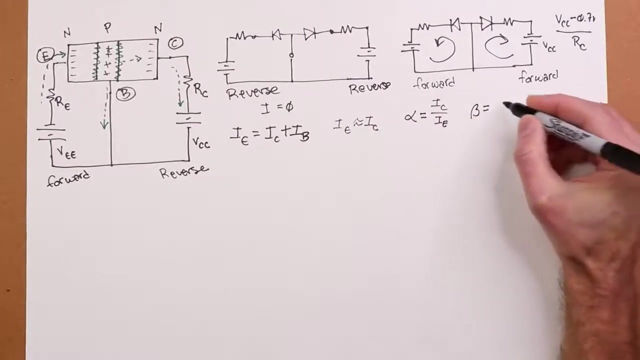 actually gets through into the collector. that's called alpha. so alpha is defined as collector current divided by emitter current. another way of defining this is between a ratio of the two exiting currents, the collector and the base. we call that beta. so beta is defined as IC over IB. right, okay. 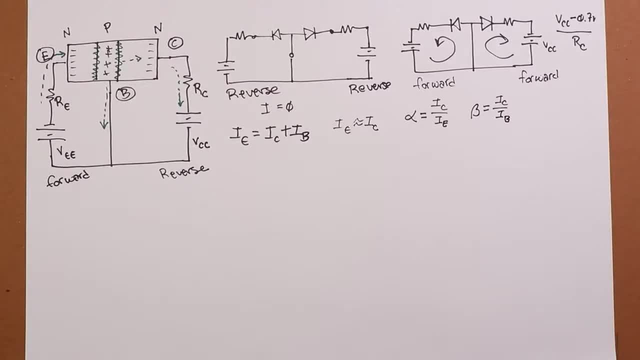 now, before we go any further, let's do a little demonstration, because sometimes people have a hard time with this idea of the electrons, sort of you know, falling into the holes and you know the percentages. sometimes it's hard to grab your mind around. so we're going to call up on an old friend, our old electron. 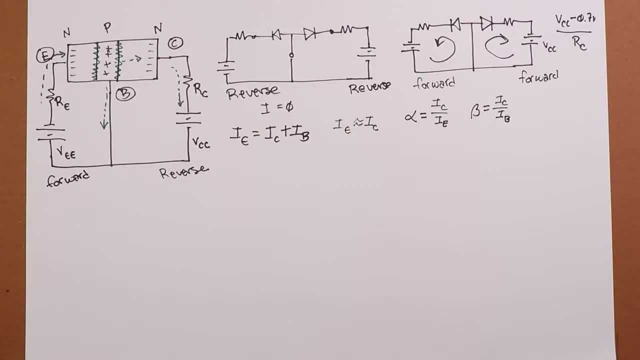 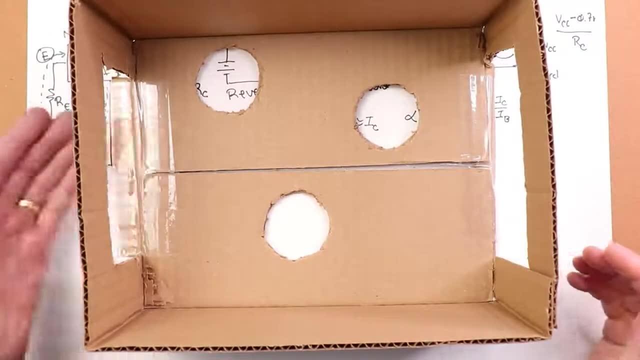 buddy, and what I've done is I've created a little sort of model, kind of a cheesy little cardboard box model of the base, essentially. so over here we have the emitter and over here is the collector. so what we're going to do is we're going 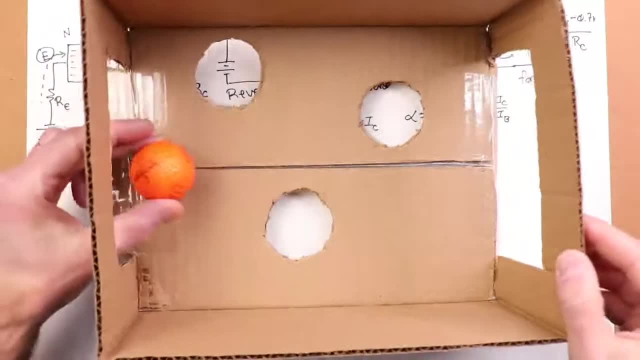 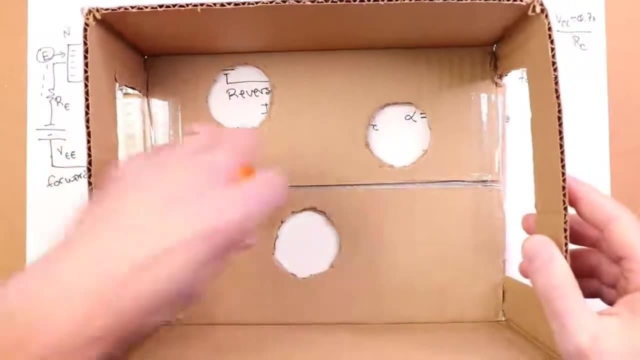 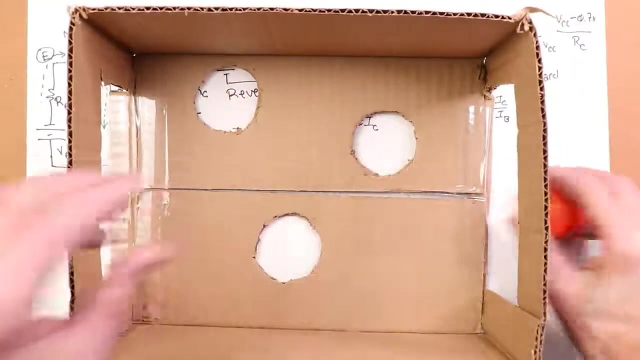 to take some electrons. we're going to pass them through here. these are the available holes literally right in the base, and the electron will come through. you know, might find a hole, in which case we have a recombination current. otherwise it's going to come through out through the collector. all right, so we're just. 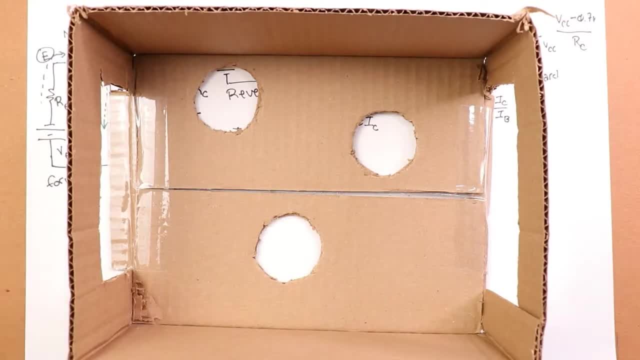 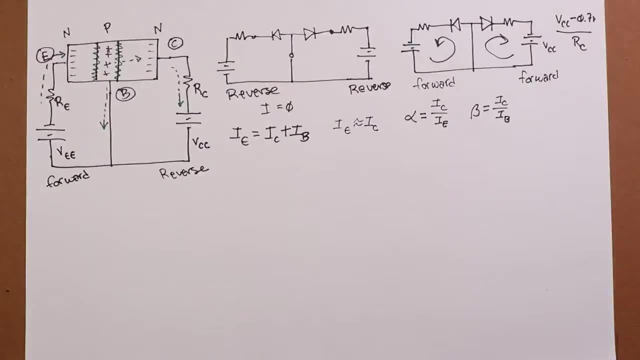 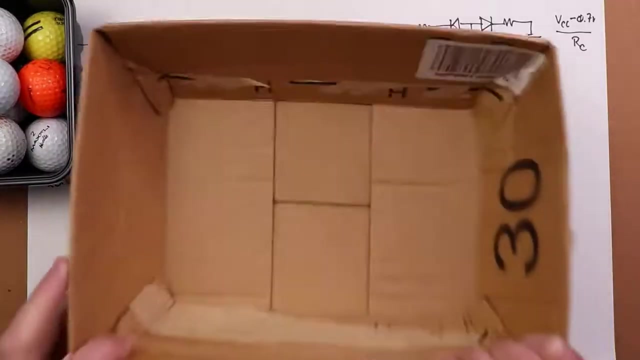 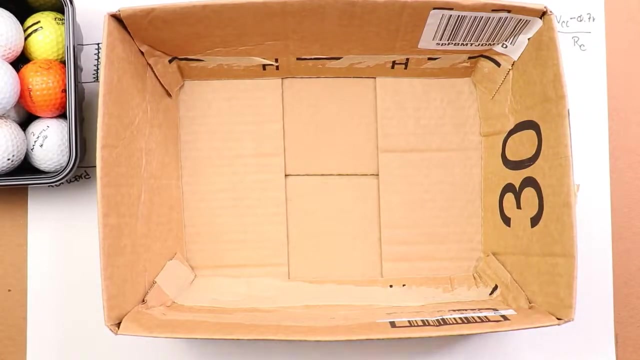 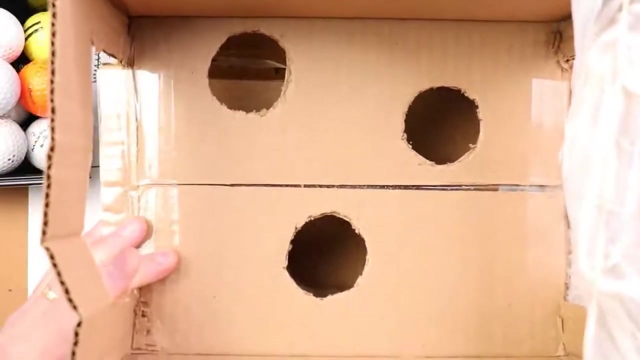 going to run a little experiment here and see you know what we wind up with. okay, all right. first, a bunch of electrons. I've got 10 of them. second, got a little box over here to hold the electrons when they fall through the holes. all right, now we have three nicely widely spaced holes and you would expect, you know just. 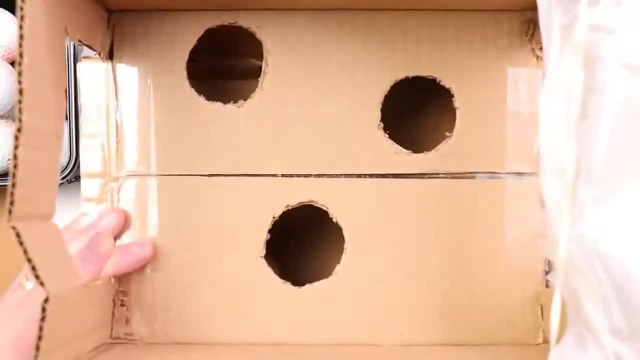 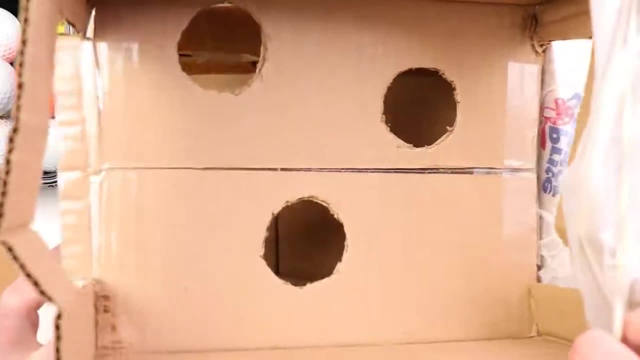 looking at this quick, you know just a lot that weapons like the first one, the first one, the third one, the third one are actually shown that a fair percentage of these electrons you know would fall into these holes. so let's find out. My little bag over here on the side so these don't go all over the desk. 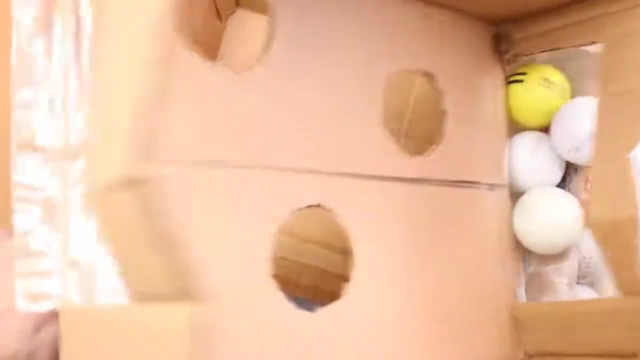 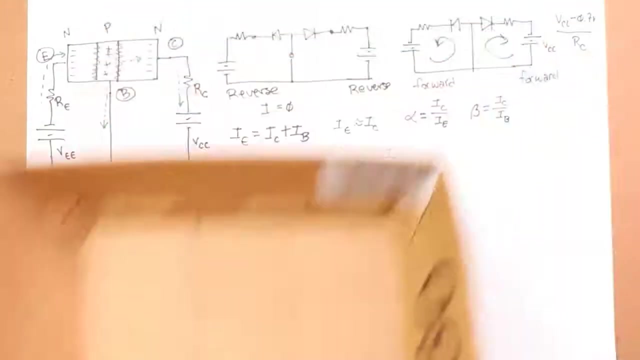 Look at that. none of them, not a single one, fell through. I write out of ten. well, if we ran this through the colder individual holes, there would actually be a fair percentage of electrons in the physical package to be able to connect everything. So my little name: pillow things over here. write it out the whole box. 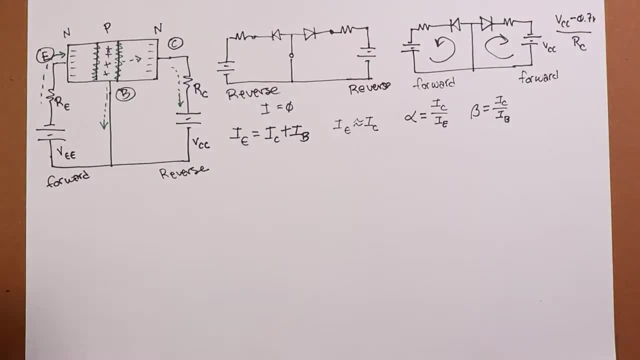 All right, All right, we want to know 8!. Let's go, let's look. 10, indeed, Let's put the first atom in mine. many times, and as you can guess, I have, you would find that you know typically. 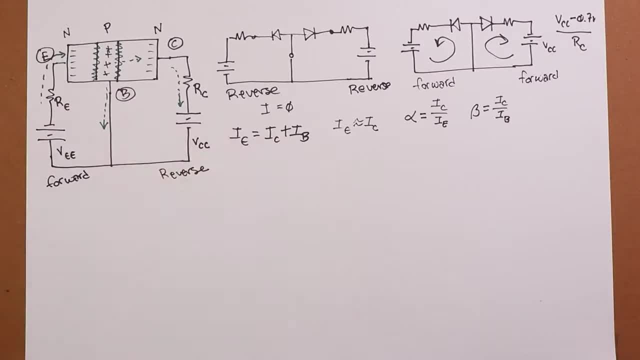 one or none would actually make it through there, Even though there's three and they're nicely spaced there simply isn't enough time for those golf balls, our electrons, to find a hole and fall right through to have just the right energy level in our analogy. Okay, So we find that you know typical values for 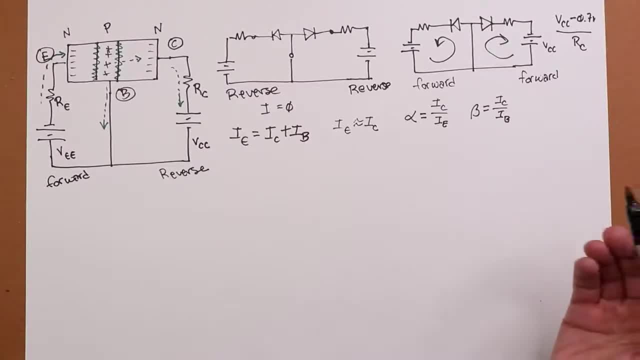 these transistors Alphas are, you know, 0.99,, 0.98,, 0.995, something like that, and those translate into betas of maybe 100, 200, something along that line. Now, 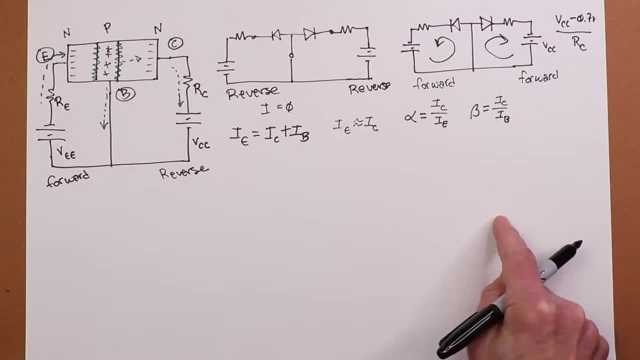 knowing one, you can find the other. It's a relatively straightforward process to do Again, if we remember Kirchhoff's current law right. So alpha is defined as IC over IE, beta IC over IB. So we could rearrange these a little bit and say that IC is equal to alpha times. 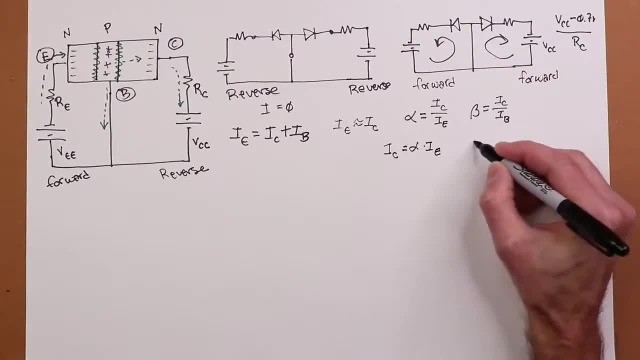 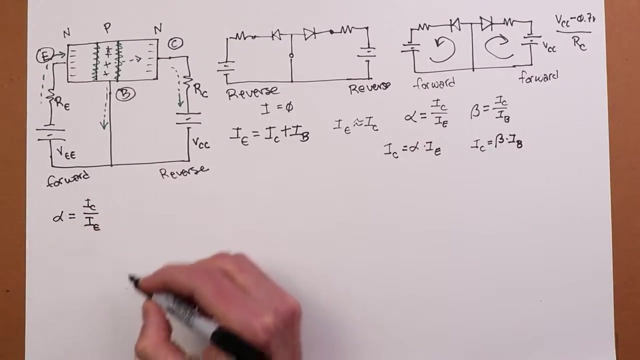 IE. We could also say that IC is equal to beta times IB. So if I look at alpha right, that's defined again as IC over IE and I'm just going to make some substitutions in here. So we know that IE is IC plus IB, but we also know that IC is beta IB. 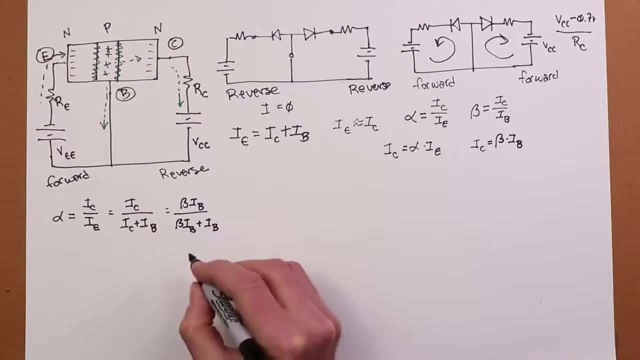 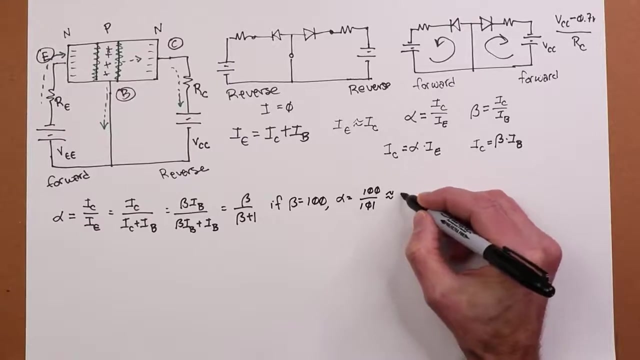 and I can factor out that IB down here, and we would find that alpha is equal to beta over beta plus one. So if your beta was 100, right, then your alpha is 100 over 101.. In other words, just a shy bit over 0.99, right. 99% of the injected electrons are 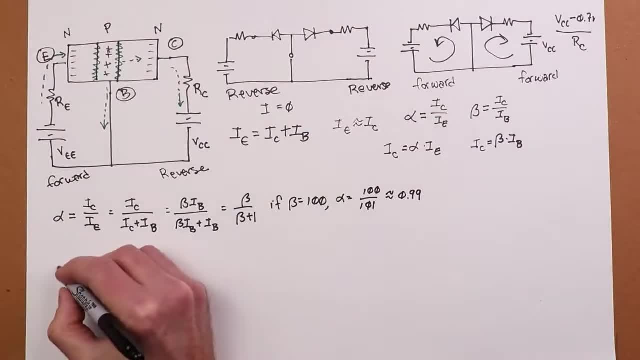 gonna wind up in the collector. Similarly, we could look at beta. Alright, so beta is IC over IB and IC we know as alpha IE. IB can be written according to Kirchhoff's current law: IE minus IC. Okay, So IC again, alpha IE. 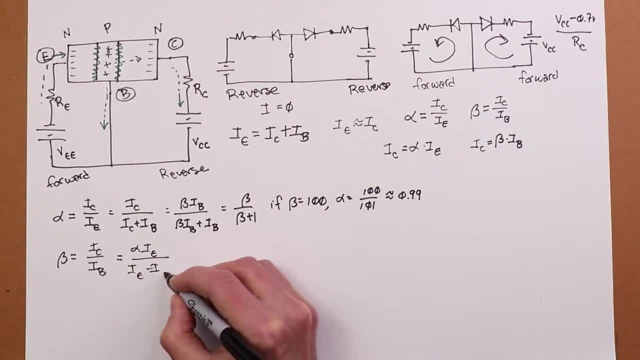 and then IE minus IC. Okay, So IE minus IC, and then IE minus IC, and then IE minus IC. Okay, So I see again alpha, IE, And now you can factor out your IE values and you find out that beta is equal to alpha. 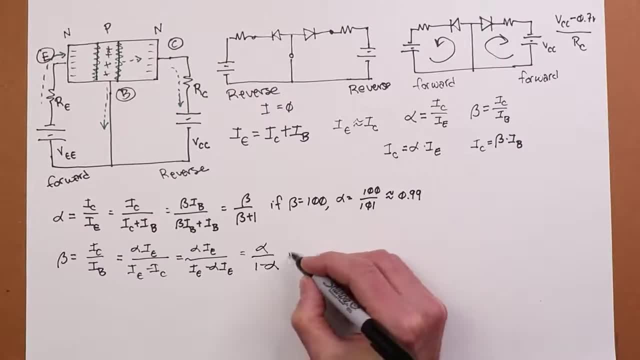 divided by 1 minus alpha. So if you had an alpha of, let's say, 0.98, 98%, then beta is 0.98 divided by 1 minus 0.98, which is 0.02, or a beta of 49.. 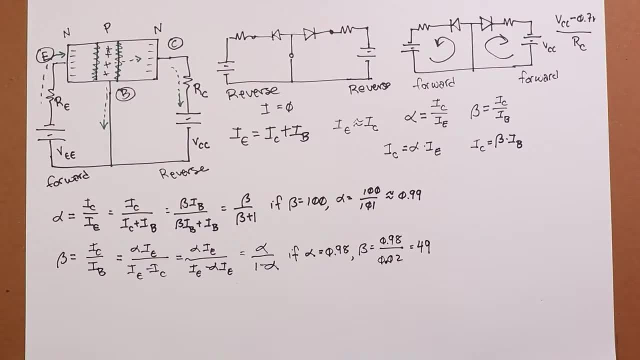 All right now. practical end of this. Very often we're going to use the base as the input and then the emitter collector as the output. Now remember the green over here. that's electron flow. That's why I did it in dotted line. 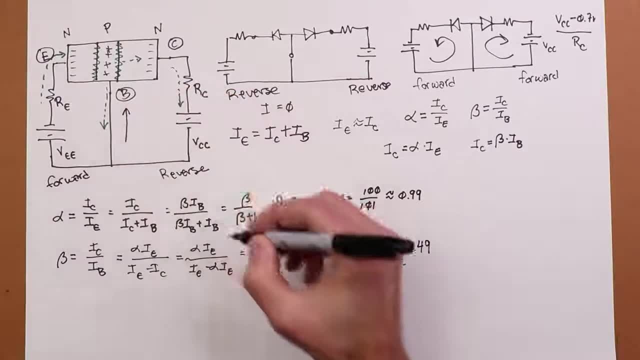 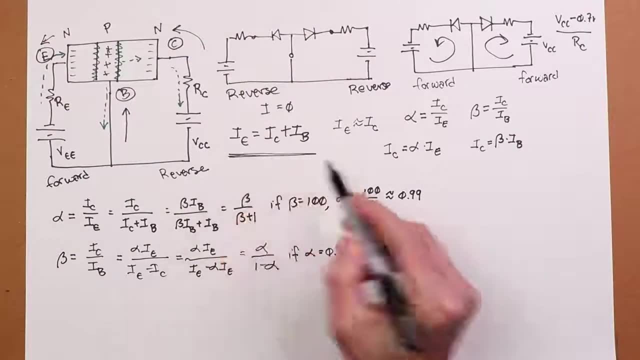 Conventional flow. current goes into the base, into the collector, out of the emitter. This still works, KCl still works, But that's conventional flow. So typically what we do is we control the base current and that acts as kind of like 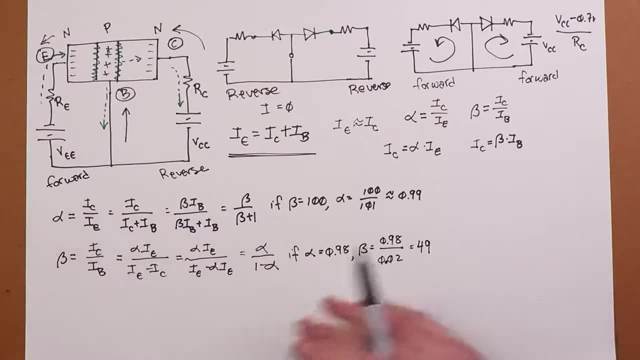 a lever amplifying the current characteristic, essentially this right here. So we can make a little model. If we think of IB as the input, sort of the little part of the lever that we're going to push up and down, the collector becomes the output. 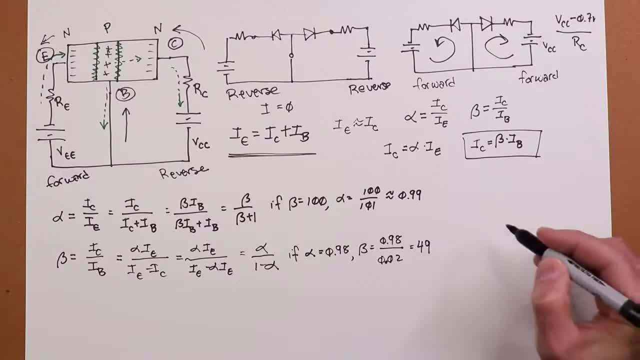 So we make a model, a very simple model, for our transistor that relies on a current-controlled current source, a current-controlled current source, And it looks something like this: All right, Cool, We have our collector up here, emitter down here, base back here. 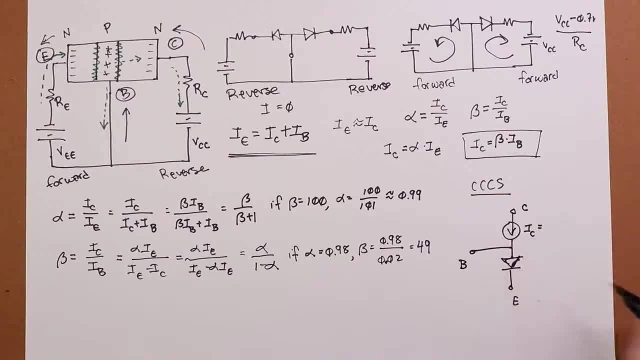 The value of this current source right- this is IC- is simply equal to beta times IB. So we put in some base current, There is a beta value, maybe 100, 200, whatever it is that amplifies up, whatever the base. 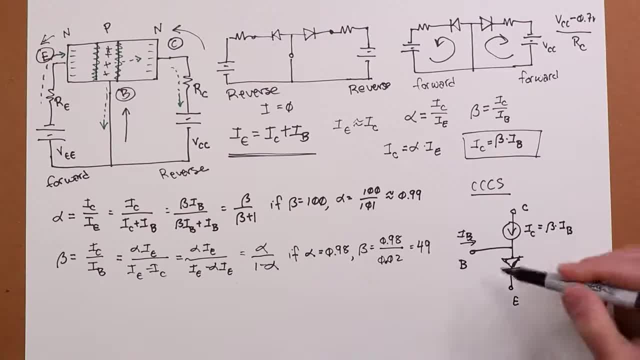 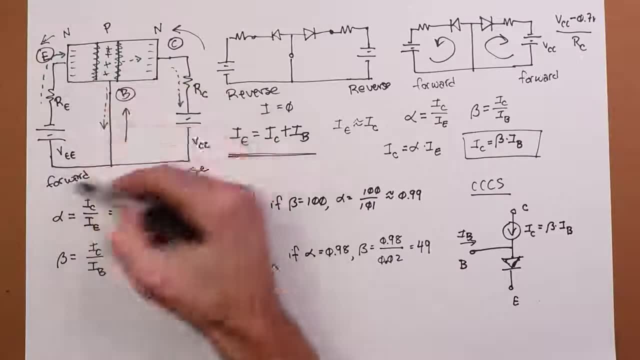 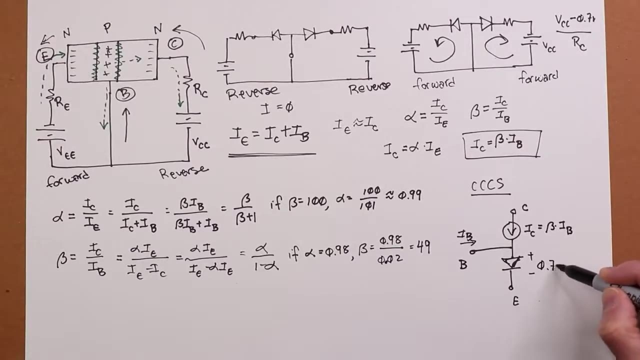 current is And that produces a big collector current. And for our bias calculation we just consider the base emitter as the forward-biased diode. Remember the emitter base is forward-biased, So this we can approximate as about 7 tenths of a volt. 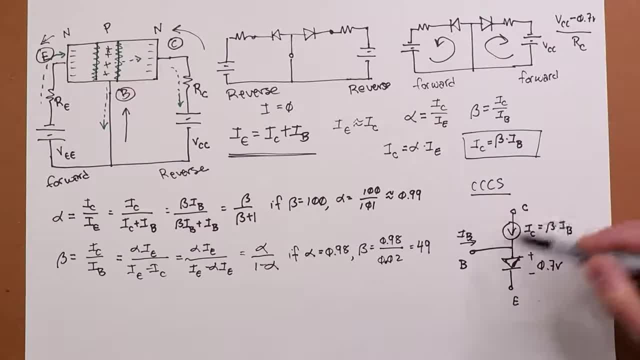 Call it a day. So the voltage from collector to base? we don't necessarily know like this, because that is, of course, a reverse-biased diode. So what is that? That's going to depend on what the surrounding resistors and power supplies and so forth happen. 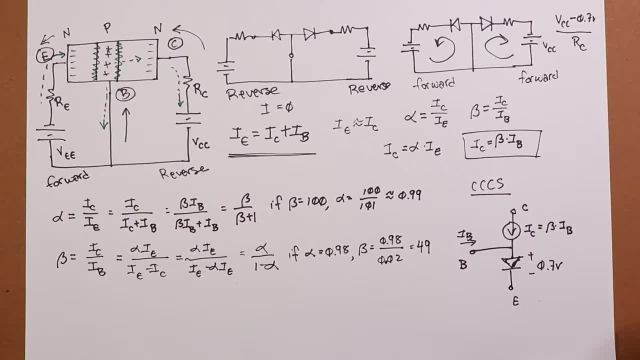 to be Right, OK. So typical numbers for beta small signal transistors: 100, 150,, 200, maybe 250.. For power transistors, because they're, you know, beefier, not quite as high, you know. 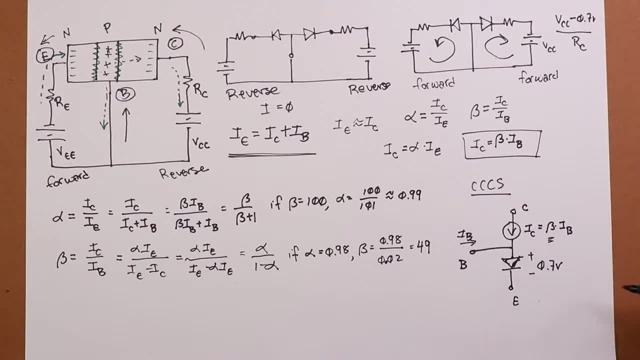 maybe 50, something like that, 30,, all depending. OK, Next time what we're going to do is take a look at some device curves. Right, As we vary voltages and currents. what kind of characteristics do we get? 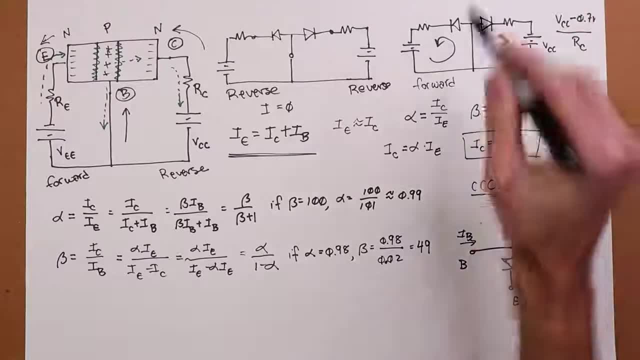 Right, We've done this for diodes. We know the typical diode curve. that's where the 0.7 comes from. So what actually happens with our bipolar junction transistors? See you then.